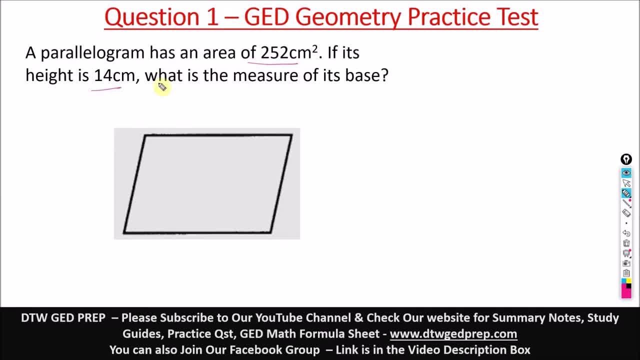 this. Okay, if its height is this, what is the measure of space? now, from our formula sheet, you don't need to cram the formulas because you are given the formula sheets would be given to the formula sheets, it would be on your dashboard, So you don't need to memorize any formula. Okay, so from our formula sheet, the area of a parallelogram is a is equal to base times the height. Okay, base times the height of the parallelogram. Okay, this would be the height. 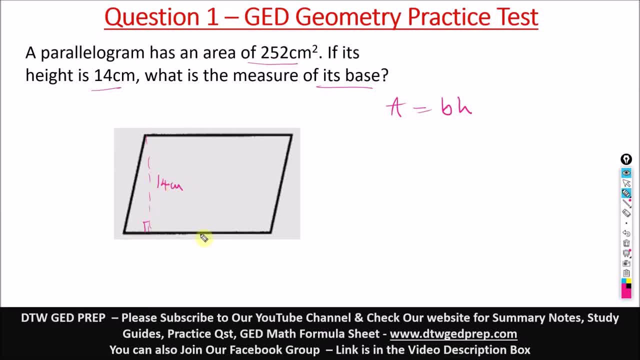 All right. so if the height is 14 centimeter, what is the base? and we've been given the areas this. so you put for a, a is equal to 252.. And our height, h is equal to what? 14 centimeters. So let's put this here. So a is this, you know, just substitute. we're looking for b. b is unknown because b is unknown, that's what we're looking for. times your h. you know, b and h, what? 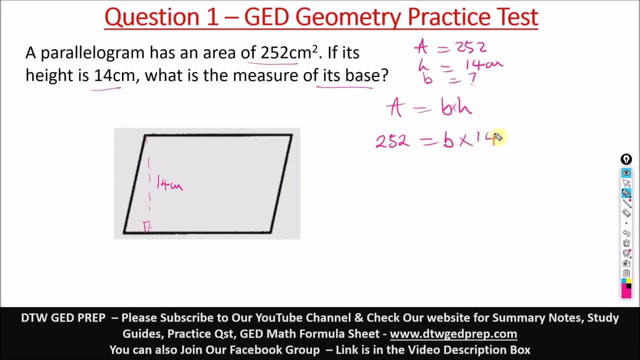 b and h. what binds them is what multiplication, so times what 14.. So to get b, we divide both sides by what? 14 divided by 14.. This 14 will be canceled out. we're left here with just b, and 5252 divided by 14 is 18.. Okay, so b is equal to 18 centimeter. okay, because here we have centimeter square And here we have just centimeter. one centimeter will cancel out one centimeter. we're just left with one. 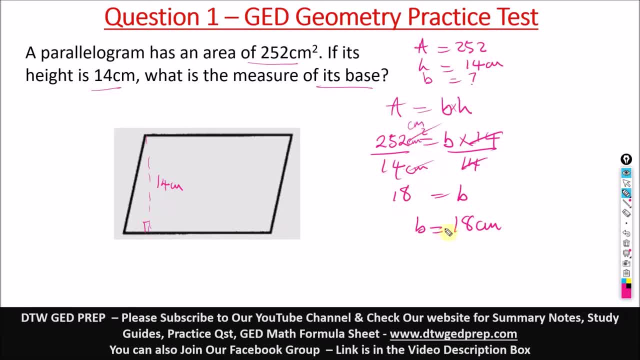 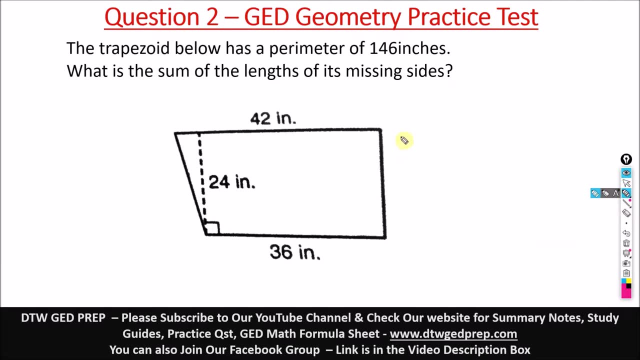 centimeter, we're just left with one centimeter. that's why we have b is equal to 18 centimeter, so our base is 18 centimeter. on this question, let's go to the next one. okay, question two of the ged geometry practice test says the tripezoid below has a perimeter of: 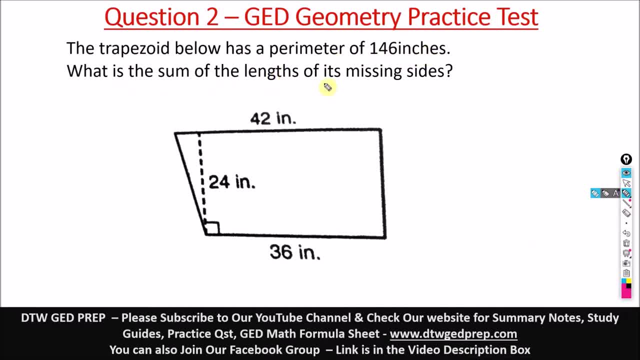 this: what is the sum of the length of its missing sides? okay, when we talk about perimeter, perimeter is all about the summation of all sides of any shape, whichever shape it is. is the summation of all sides? okay? so it says: the perimeter of this is this: okay, so p is equal to. that's the perimeter. 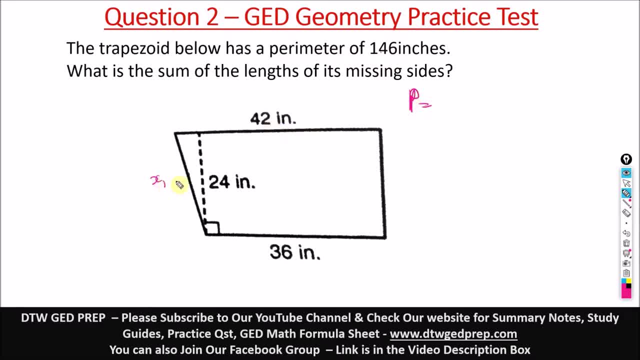 p is equal to. let's give this unknown side as x1 and x2. okay, so we have here. we can just put: the known sides are 42 plus 36. then plus the unknown side, that was x1 plus x2, and we've been told that p is 146, right? so we have 146 equal to this plus this. 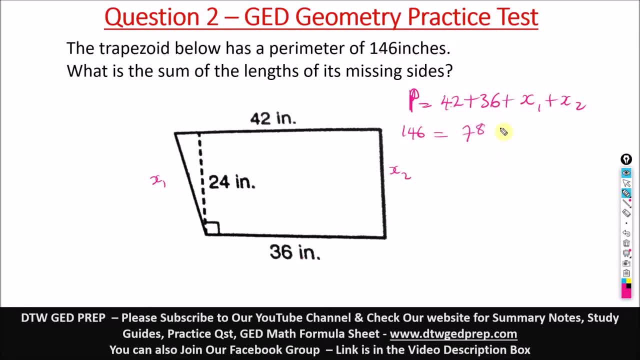 would give us 878. okay, plus x1 plus x2. so to get x1 plus x2, we take this here, so we have 46. when you're taking a number over to the other side of the equation, it becomes: because here it's a positive, when it crosses a sine. 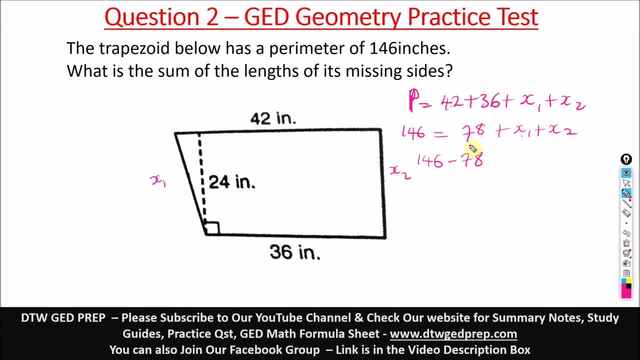 changes to what negative. or you can say: subtract 78 from both sides. okay, either way, okay. so here, 146 minus 78 will give us what 68 equal to x1 plus x2. so here our answer, because it says what is the sum of the length of its missing side. so the sum of the length of the 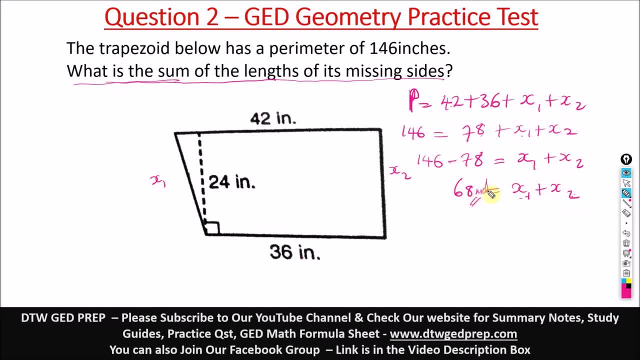 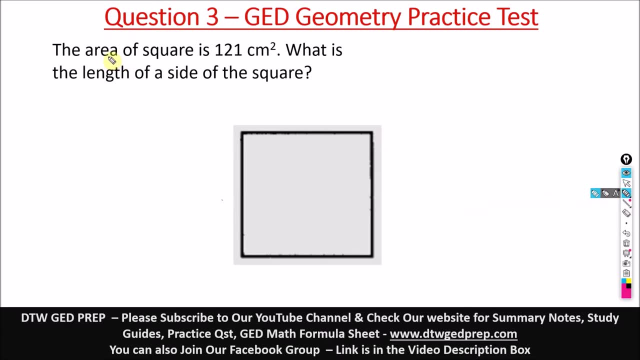 missing side is what? 68 inches. don't forget the units, inches. okay, so this is the answer for question two. let's go to the next question now, question three of our gd geometry practice. it says the area of a square is this: what is the length of a side of the square? length of a side? you can see a side, okay, and from our formula sheets, 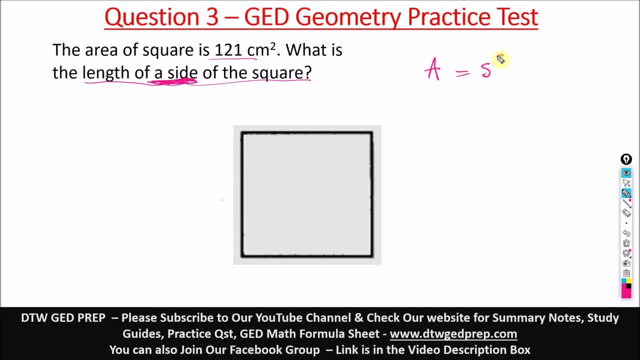 the area formula for area of the square: is the area of the square, is the area of the square, is what s square? okay, and it has told us that area is what? one, two, one, one, twenty one. so what? to look for the length of a side? that's one side s, okay, all right, you know a square has all sides. 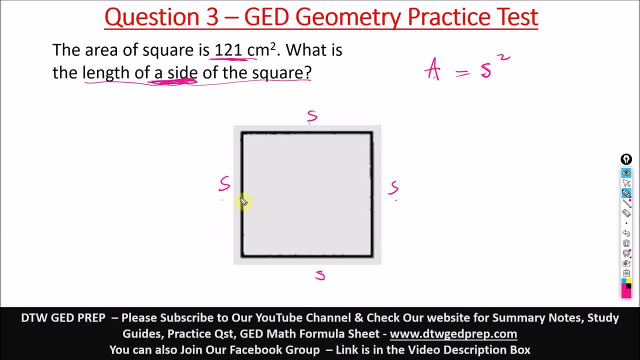 what's equal. so if this is s, this is s, this is s and also this is s okay. so one side, all sides are equal, so what you just look for s alone. so here, the area of the square is what s square is okay. of this square, is one, two, one equal to s square? now, when you have something like this in maths, 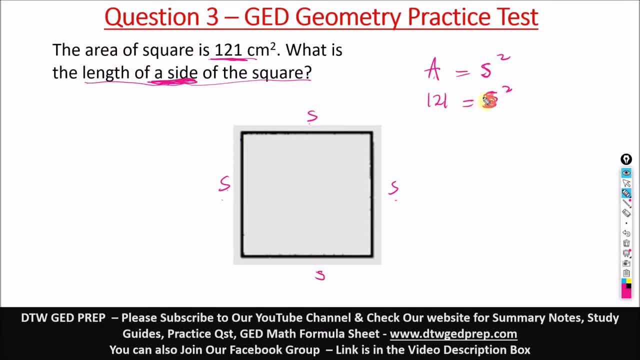 s square and you are told to just find only s. what you do is you square root both sides- okay. when you square root s square, it's just going to give us 1s, okay. and when you square root 1 to 1, 1 to 1 is going to give us 11, so s is equal to 11 centimeter. all right, do you get me? 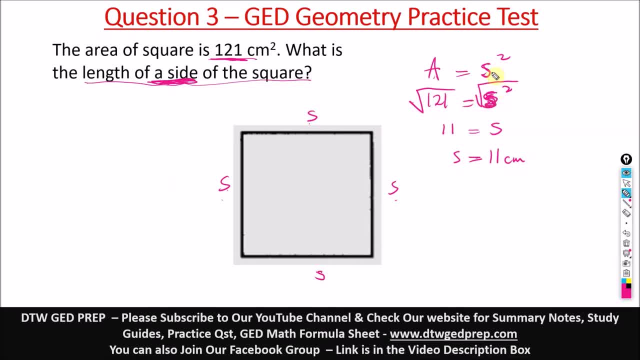 when you have this in math, you have s, s square, okay, and 1 and another number by the side. when you want to get just one value for s, what you do is you find the square root of both sides okay, and i think i've explained this. 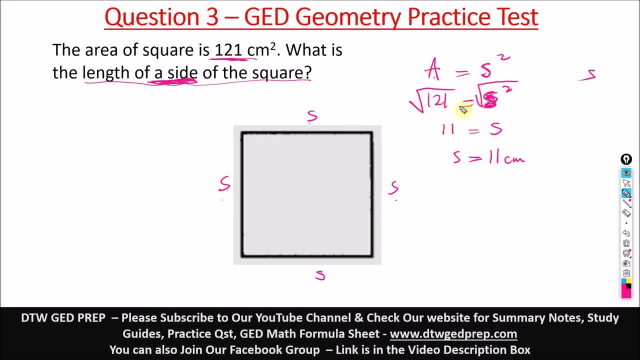 it in a separate video which you can find on my channel. okay, if i've not, really, if i've not done that, um, i'm going to check and do do this. i've explained these powers after this video, okay, but this is what you do in maths, all right. so when you have something like this, you are just to find only. 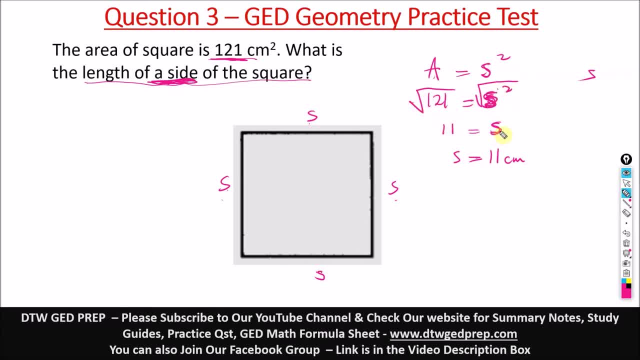 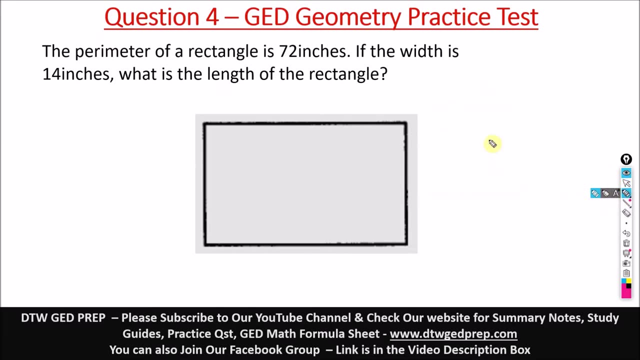 s your square root, both side. so you find the square root of this. it gives you as the square root of one to one, it gives you 11.. so our answer is: what's 11.? this is the length of the side of this square 11.. let's go to the next question. number four says the perimeter of the rectangle. 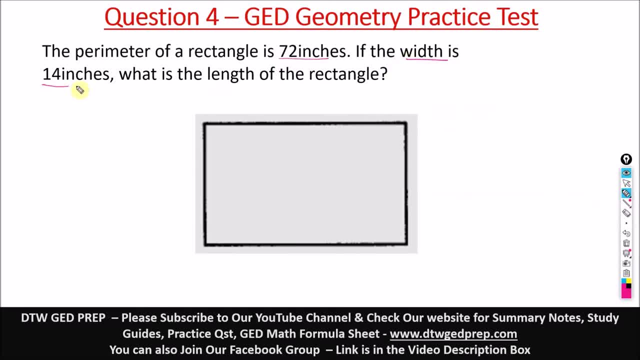 is 72 inches. if the width is for 14 inches, what is the length of the rectangle? so the width is 14 inches inches. the area, that's the area is what the perimeter i mean perimeter is about 72 inches. so what is the formula for the? 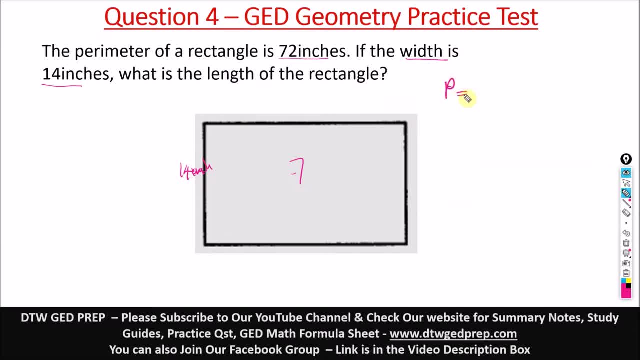 perimeter of the rectangle. it is p. from our formula sheet, p is equal to 2l, that's 2 times the length plus 2 times the width. okay, from here we know that p is 72. we don't know our length, so let's put it. let's leave this as 2l plus we know our width as 14. that would be 2 times what, 14.. 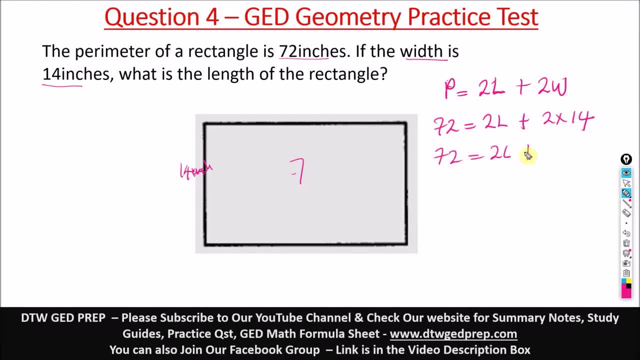 so we have 72 equal to 2l, plus what is 2 times 14, that's 28. take 28 here, okay, and leave just 2l here. you know we're looking for l. take a 28, here we have 72. taking a positive 28 down here, it becomes a negative 28 equal to 2l. and what is 72 minus? 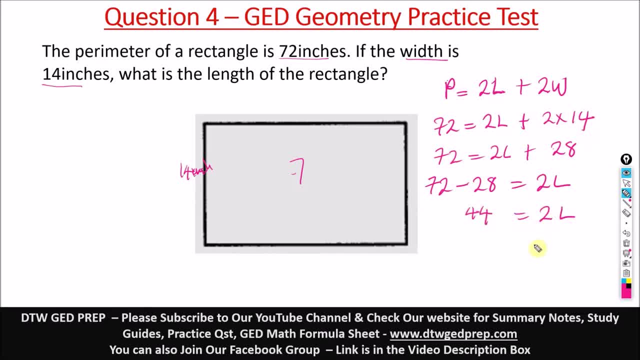 28, that will give us 44, equal to 2l. now to get l. you know this is uh, the is bounded by multiplication sign. okay, so to get l, what we do is we divide both sides by two, so two would cancel out here to just leave us l alone. and you know, whatever you do to one side of the, 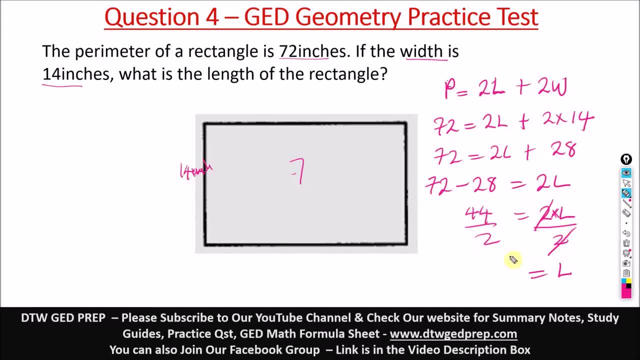 equation you also do to the same. okay, that's what i did on that um: square root in both sides. when you square root one side, you have to square root the other side. okay, so 42, 44 divided by 2 will give us for 22. so l is equal to 22 inches. okay, so this is how you find your length of this. 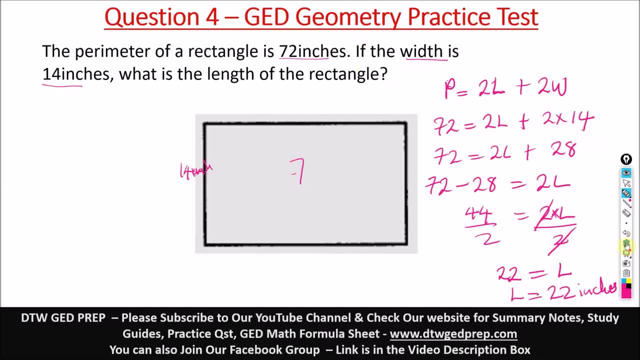 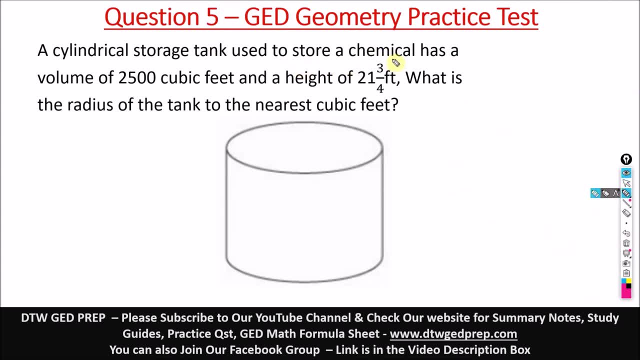 particular rectangle, given your perimeter, number four. here it says: a cylindrical storage tank used to store a chemical has a volume of this and a height of this. you can see this fraction. the gdl is putting fractions in there. so in their word problems, their geometric problems, you know. just to test your knowledge of fractions. 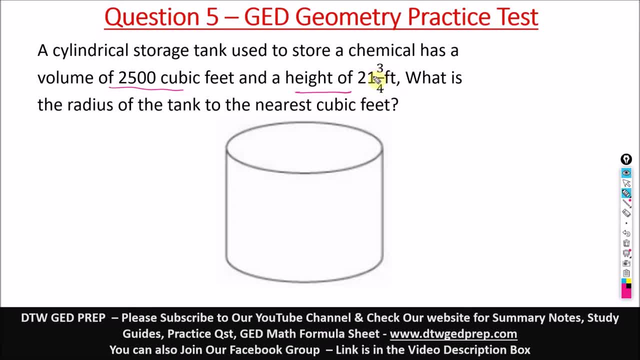 you might not really just see fraction questions given directly. they'll just be in your question as word problems. so you should know how to you know work with fractions. and the best thing about um, the gdl, is that the fractions given can be easily converted to your decimal. 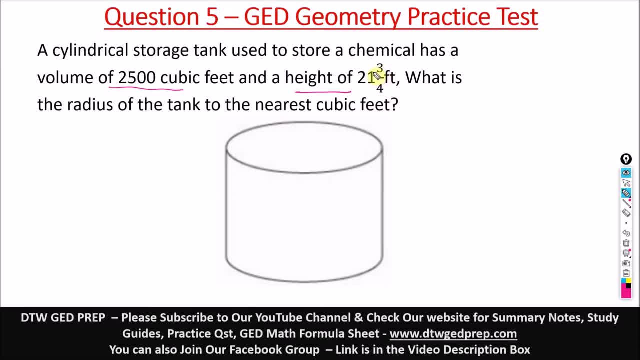 points. okay, i mean your decimal figures, all right. so these three over is always good to know. know some similar fractions and their conversion to their decimal uh numbers. okay, three over four is 0.75 and one over two is what? 0.5? okay, these are the popular. 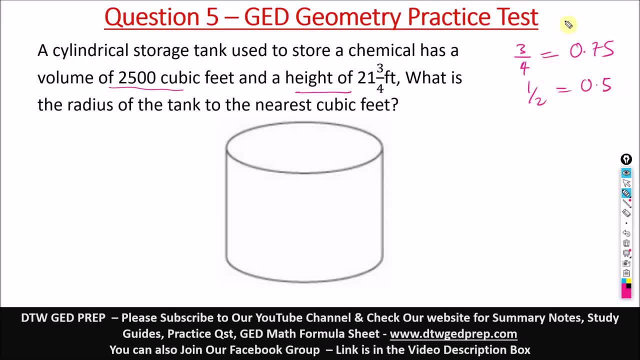 ones, um, that usually come out from the ged test, so you should, you know, get to know them. one over three is 0.33. okay, this is 0 point, sorry. at the end of the five. okay, 0.50, okay. so notice how easy the siri dressing of represents this nike and say so themselves. over a number is o slowed on a. score of four and no53, and this means we're going to add alsoож, so over three, we are left with what we would anmolcıothers, and they are said to be that 0 protective by 123. okay, this is slick, forgetting number overatorio. i have not even counted two measurements. 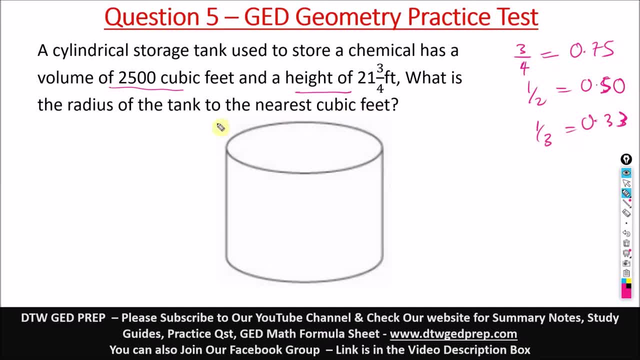 but for me, that is what the jiri measure of f, let's go back to the number, and here you're memang bring out to the easy conversion from fraction to decimal. okay, so from here now, you see, we're given the volume, we're given the height and we're told to find the radius of the tank. okay, that's what we're. 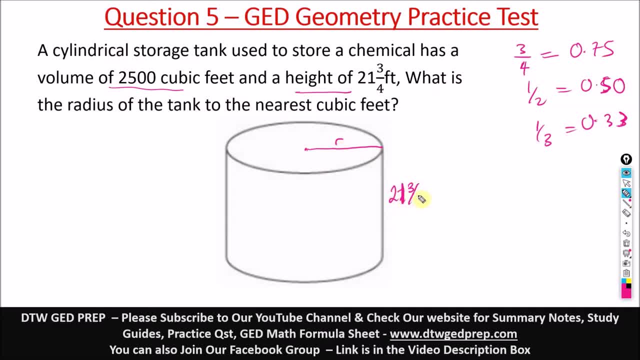 told to find the height is what: 21, 3 quarter. we're told to find the radius, the volume is 2500 cubic feet. okay, so from our gd formula sheet, if the volume of a cylinder is what by r square h, all right, we are given our v as this. so let's put this, put it here: 2500. 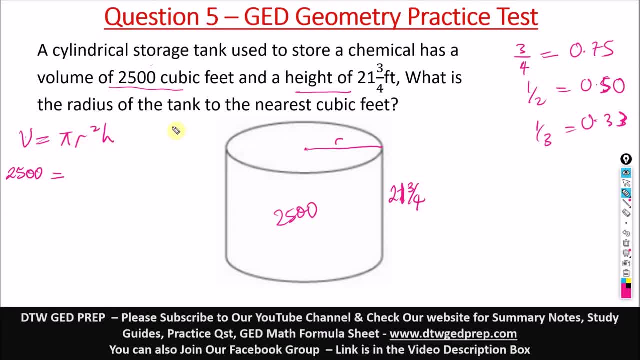 our pi from the gd. it would always state pi as what: 3.14. so we have 3.14 times. we're looking for r, so we leave r as r square, since we don't know r times. h is what 21, 3 quarter we can. 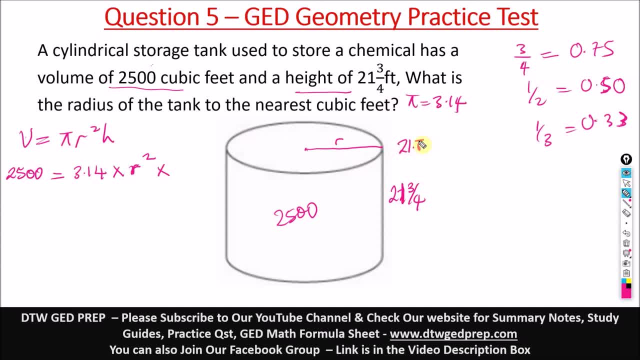 quickly change this, as what you can do is just add this: 0.5 to 21. okay, 0.75 to 21. when you add it, you have 21.75. okay, so we have 21.75, all right. so what we do here is: i would prefer that we multiply this. let's. 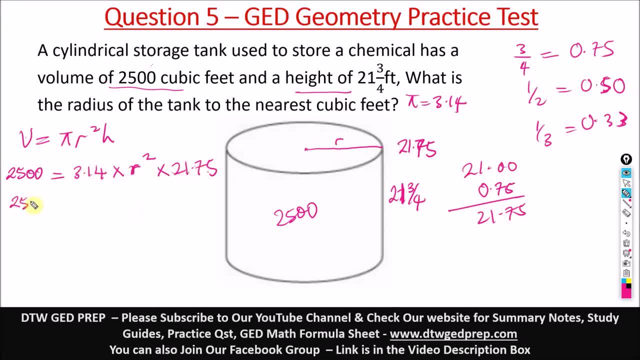 multiply these two numbers here, so we have 2500, equal to this times, this times, this times this, and give us a 68.295 times r square. now to let r square be alone here, so we can find r with the variable size by 68 295, by 68 295, and this would cancel. so we're left only with 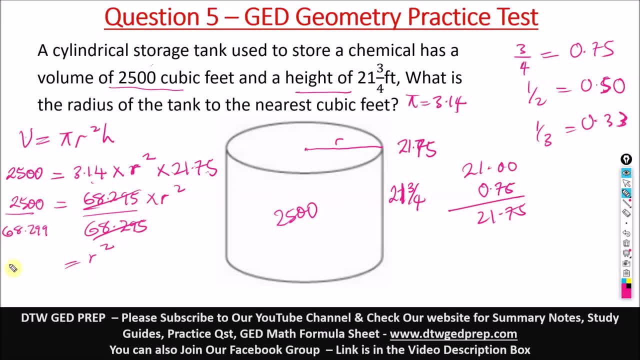 r square here. this divided by this would give us pointing your calculator. there's a calculator. um, there will always be calculator on your dashboard for questions like this calculator will be allowed. okay, so we have this. so it means r square is equal to 36.60 and it says: 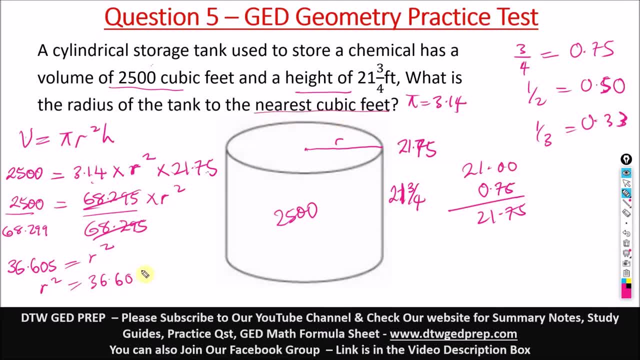 to the nearest cubic feet. so we're going to you know approximate very soon. so here, as i said earlier on, we have r squared, so to get just r alone we have to square root this, and when you square root one side, you have to find the square root of the other side, and so the square root of 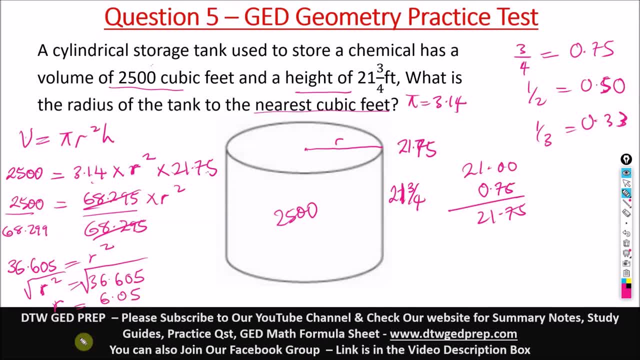 this is 6.05. okay, so from here we're told to um. what is the radius of the tank to the nearest cubic feet? so to the nearest cubic feet, r will be what the next cubic feet? that is a whole number. you look, you look at um. after, after the decimal point, you check for the next number is this: 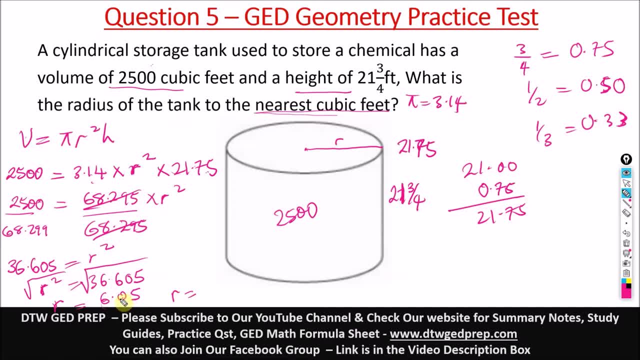 number up to five. it's not up to five, okay, so it means we cannot approximate a one to add to this six. okay, that's the way approximation is done. okay, so we can. just we have to just leave six alone. so r to the nearest the radius, the nearest um cubic feet, is what six? what? sorry, this shouldn't be. 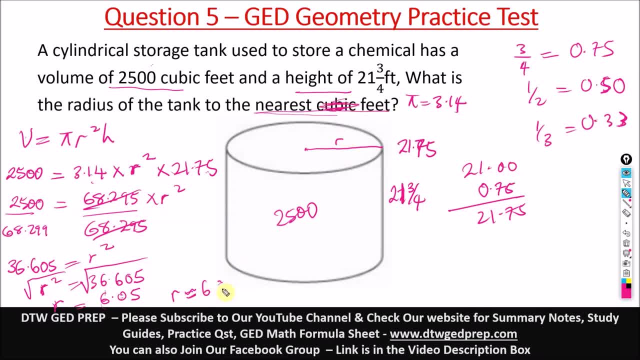 cubic feet, just the nearest feet is six. what feet? okay, so this is, uh answer, six feet. all right, you see questions like this. it might not. um, you know, did you read questions like a lot of text to get you a bit worried and confused? because all you need to know is just bring out what you need. 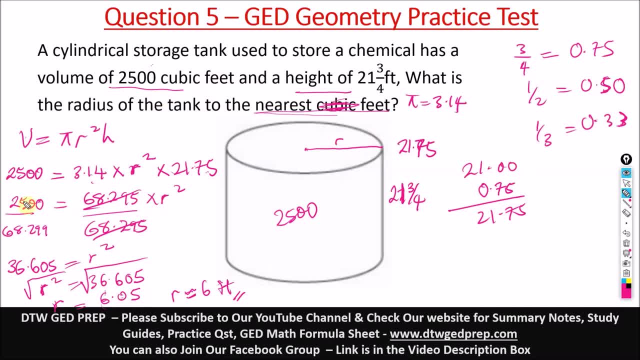 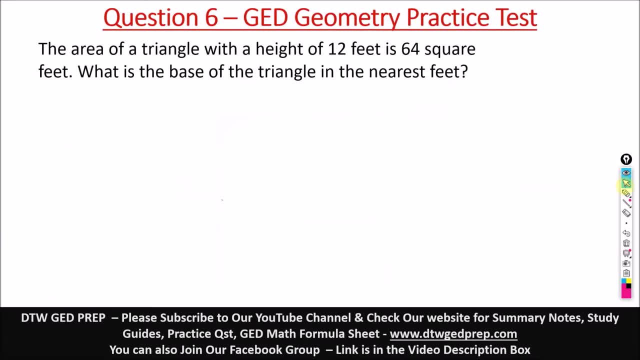 okay, the values you need. that's all, and you know. apply your formula. all right, so this is the answer for this. let's go to the next number. this question six says: um, the area of a triangle with a height of 12 feet is 64 square feet. what is the base of the triangle in the nearest feet? what is? 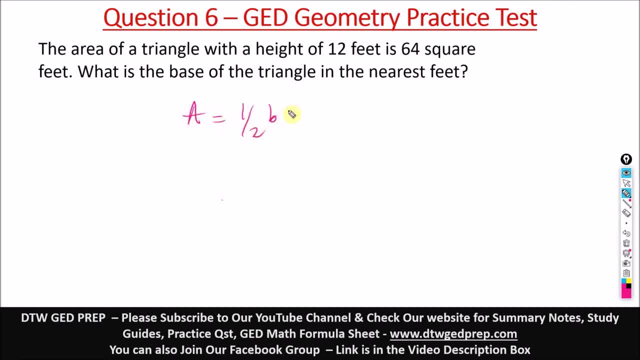 the formula for the area of the triangle is: what's half base times what height? okay, so we've been given the area as what? 64 square feet. so we have 64 equal to half. we've been given our height. we don't know our base. we're told to find the base. okay, so b times our height is what? 12? okay, 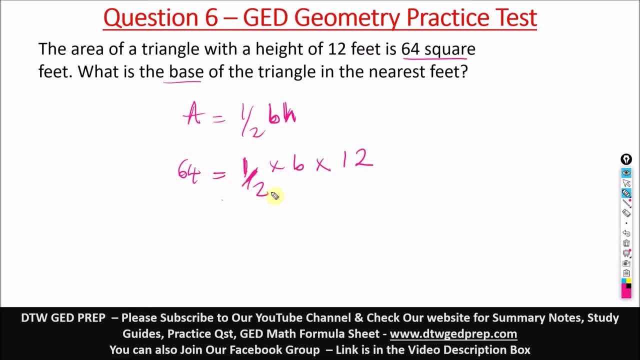 so what i'll do here with this fraction, this half, is to just say: um, i can just cross this here or i can simply cancel it out here. so i'll say: two here one, two here six. so here we're left with 64, equal to b times what six, right? so to get b, we divide both sides by six. this would cancel we're. 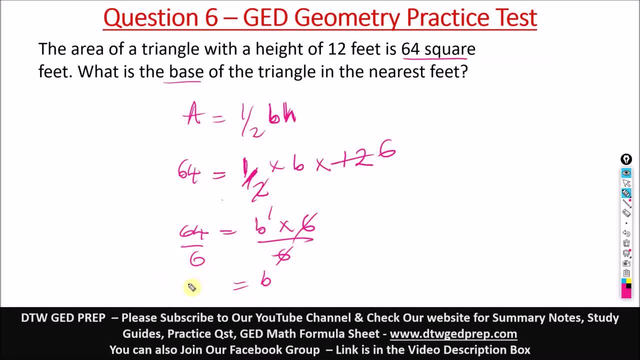 left. with b here and 64 divided by six, we'll get what? a 10 point six six. okay, so b is equal to a ten point six six. but here it says to the nearest feet. okay, to the nearest feet means we're looking at the whole number. okay, so we have ten here. 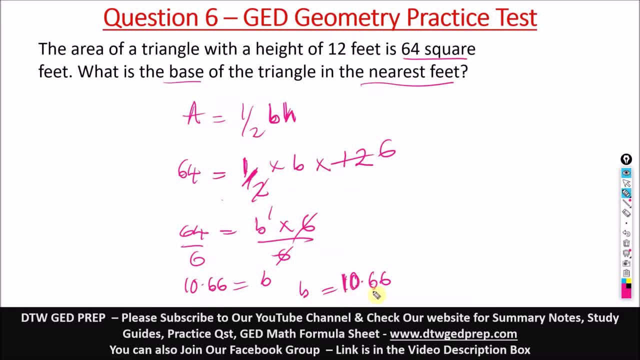 immediately after the decimal point. is this number greater than five or equal to five? it is greater than five, so it means we can approximate a one to add to here, so we finally have one plus this then will give us what 11.. okay, so to the nearest feet, our base is what 11 feet. do you see that? okay, this is our answer, okay. 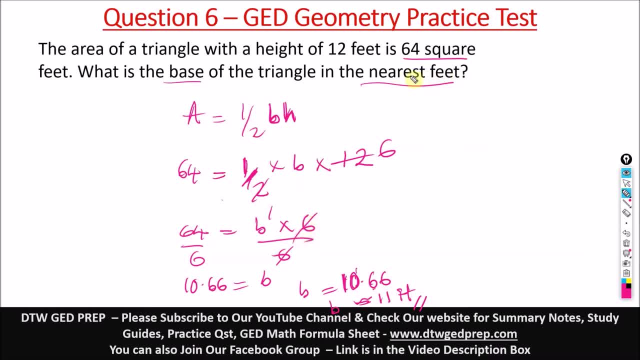 most well. i've noticed most utility questions. you always see to the nearest feet, to nearest tenth of feet, to nearest hundred of something you get. so you need to know how to approximate correctly. all right and- and most of them usually do. you know you have a box, you don't have options. 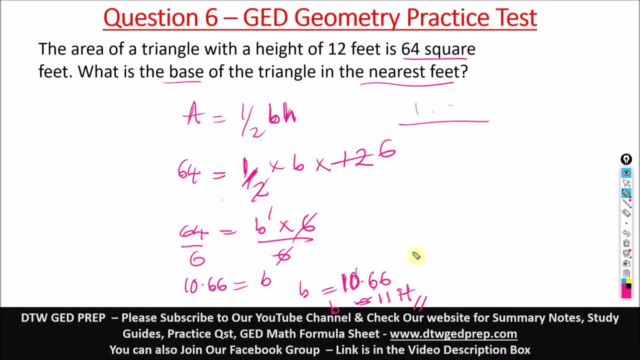 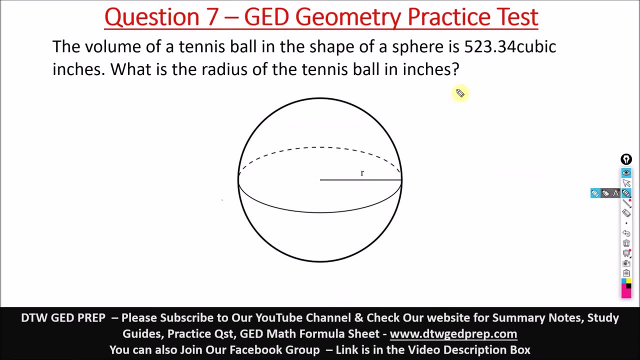 you just have a box that you have to write the answer. all right, so please, when you have that, please make sure you write your feet, okay, your unit of measurement and approximate well, okay, so number seven. we have a question here. it says seven of the ged geometry. 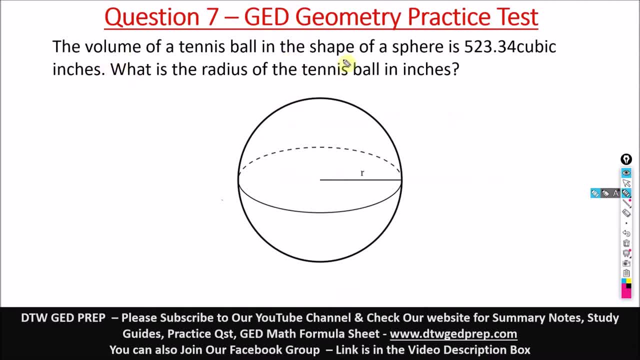 practice. it says the volume of a tennis ball in a shape of a fair is this cubic inches? what is the radius of the tennis ball in inches? so we're looking for the radius. we know the volume of the fair, all right, so we apply. what's the? 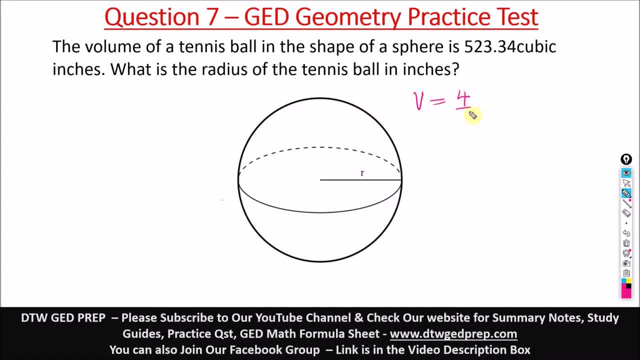 formula for the volume of the face, v is equal to 4 over 3 by r cube. okay, so we're looking for the radius. we know v as what 5, 2, 3.34. okay, equal to 4 over 3. pi is what 3.14 then times r cube. 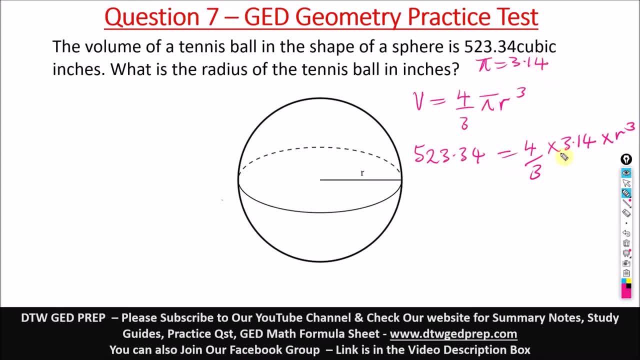 pi will always be given as 3.14. okay, you'll see it in the in the question, and the your ged formula is the diagonal and the diagonal and that's the figure of 6.4 and 6.6, if you just do the same. 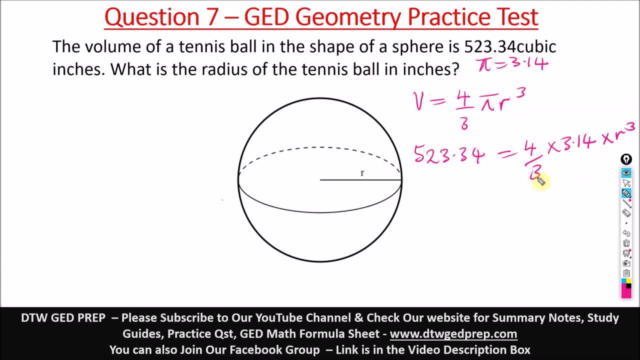 thing, you get the result in the test again, so you'll see that the estimate one is theผ2. so we have 30 and we have 3, we have 4, we have 3 and we can just multiply our number by the standard value. so the standard value of it is equal to 3.14 plus the square root, 2.3 minus the square root. 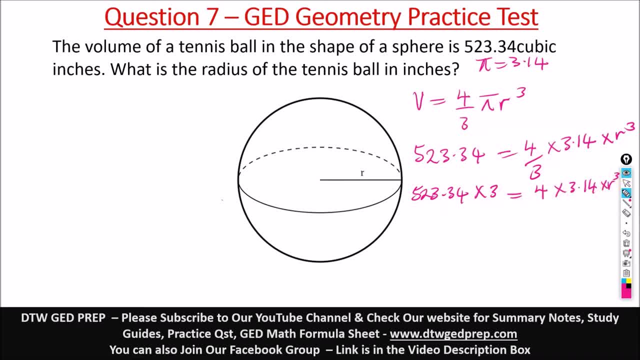 4 and we also have the diameter of what we'll do in this test. so we have the diameter of the square, 2 pi, and we'll multiply the diameter of our point square to 3.3. all right, so from here, what do i do? 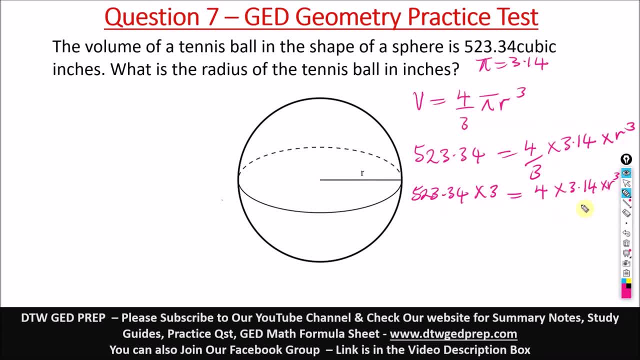 there's nothing to cancel out, so i would prefer let us just take this three. should we just take this 3.3 and arrow cube, because that's the target. arrow cube has to stand alone. all right, to make arrow cube stand alone, we can divide both sides by this: four times 3.14. okay, four times 3.14. so this would: 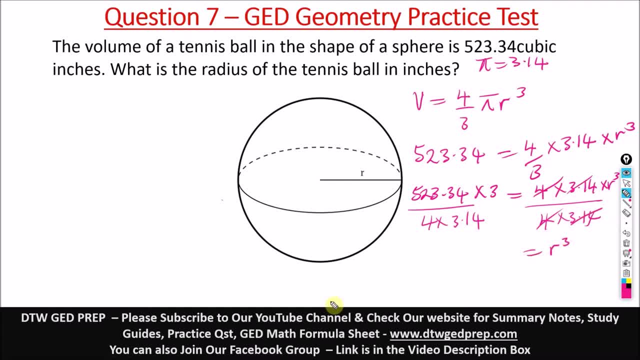 cancel out. so we're left just with arrow cube here. if you punch in your calculator, do all this- you know calculations on your calculator- you should get a 125. all right, you should get 125, and from here to get arrow alone. so this, so it's 125 equal to arrow cube, so, which also means arrow. 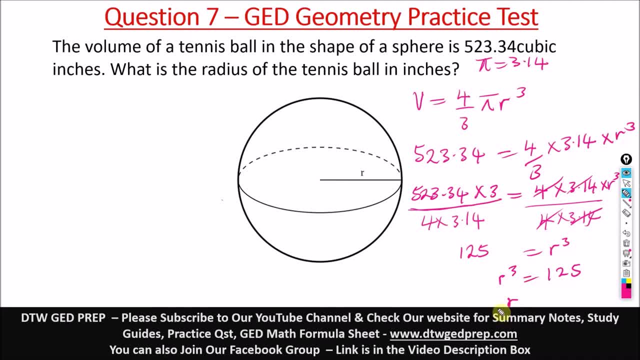 cube equal to 125. so to get arrow alone, what you do is you cube root. when you cube root arrow cube, it gives you arrow, so you also have to cube root what this um number 125 and the cube root of 125 is a five. all right, i hope you know. 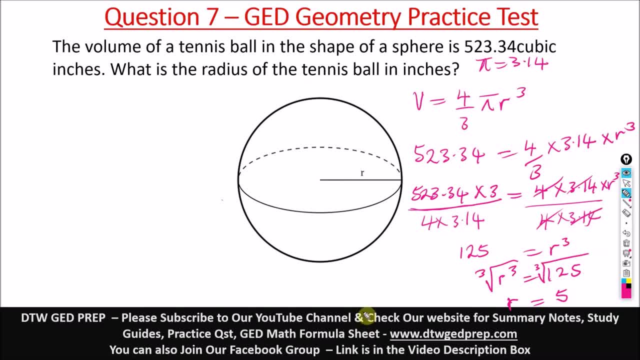 how to find cube roots. i've done a video on powers and roots. okay, you should, you should, uh, watch that video. i think i used the calculator to teach how to find cube roots and all that, so that video would help you. all right, i will leave the link in the description box. okay for you to learn further. 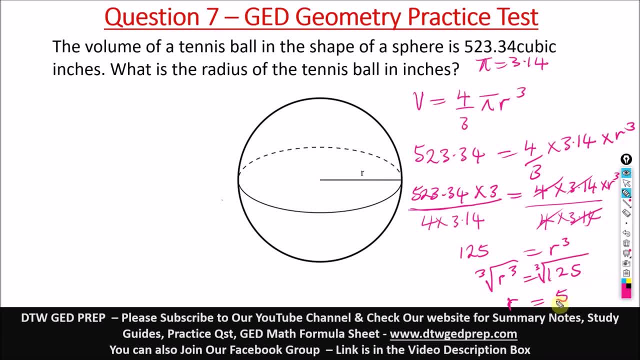 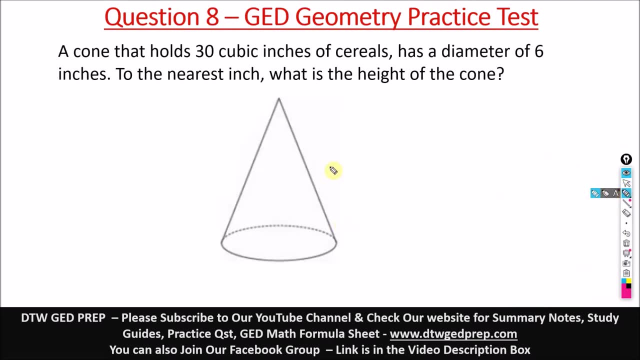 so the cube root of 125. when you use your gd calculator, you will get a five, all right. so our radius here is: what five? what in cheese? all right, let's go to the next question. our next question is a question on cone. okay, so this is question eight of the gd geometric practice test, a question on cone. 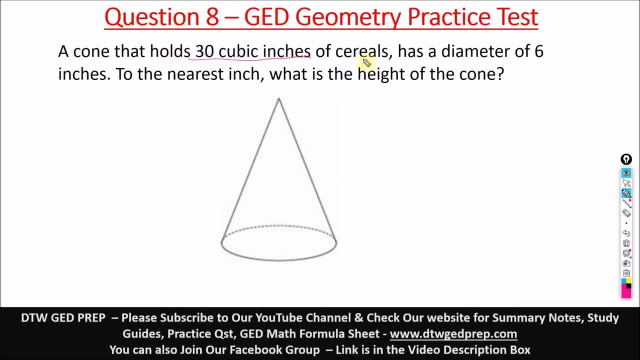 it says: a cone that holds 30 cubic inches of cereal has a diameter of six inches to the nearest square of the cone. and the diameter of the cone is six inches. what is the height of the cone? so it has it told us that the diameter is what? six inches? 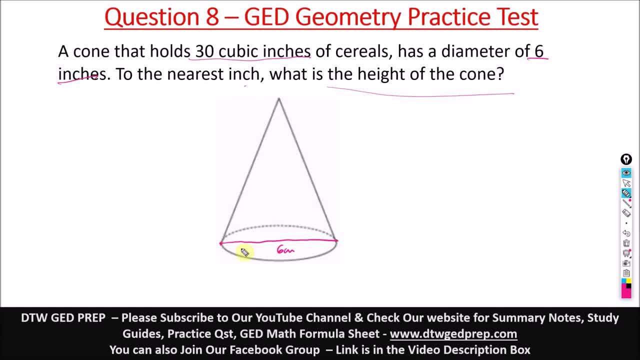 you know, the diameter is from uh, a line that crosses the center of the circle, that touches two points of the circle and passes through the center. so this is the diameter. if the diameter is six, then it means the radius, which is half of the diameter from here to here. 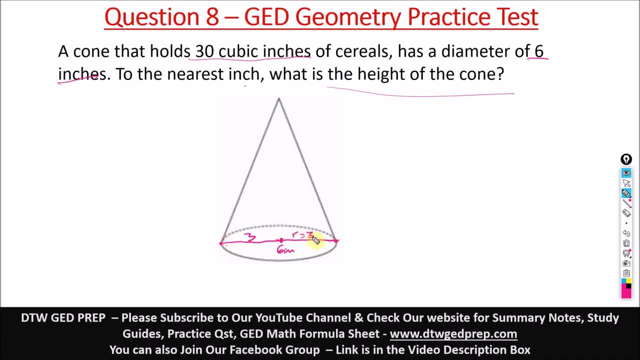 is three. from here to here is three, so the radius is equal to three. okay, and what's the formula for the volume of a cone? the volume of a cone is one over three by r square h. okay, we know that the volume is 30. v is 30 equal to one over three. 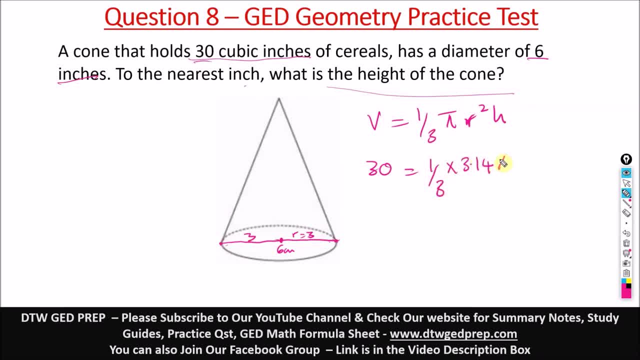 our pi is times 3.14. you know pi is what pi is- is uh, 3.14. on our formula sheet, our r square- okay, we can see. this is the height, which is d, r, then the radius is. so we will just give it the diameter now one time, okay, so here is a column. r is equal to three, so that 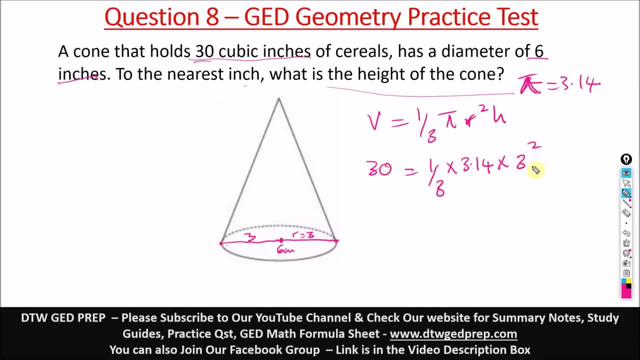 is three square. okay. three raised to the power two, then times h. we're looking for h. okay, that's the height. so from here we have 30.14.4 to the power two plus 3. could we have her times four times two? okay, that's the answer. 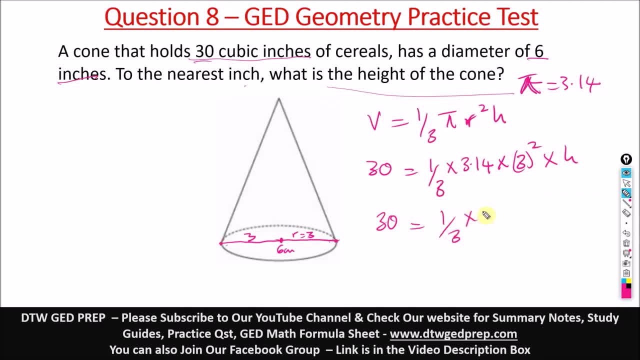 so we keep looking. we have 30 over four. we can again count the times that we calculate is equal to 1 over 3 times 3.14 times 3. square is what 9 times h? okay, i can cancel out 3 here. okay, that's uh. i'm just breaking this down for simplification, but you can just use your calculator. 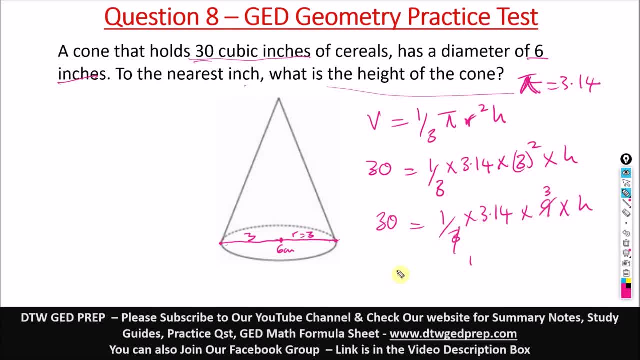 okay, so 3 will be here. all right. so from here we are left with. 30 is equal to 3.14 times 3 times h, so i will divide both sides by 3.14 times 3. 3.14 times 3- this would cancel out. 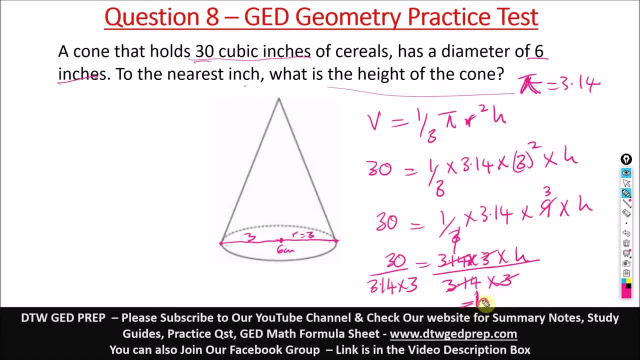 what i left just here with h, that you know. that's the goal: to make h stay alone, stand the unknown, stand alone on one side of the equation. when i do this on my calculator, 30, divide by this, by this, okay, what i will get is what? a 3.18? all right, so h is equal to 3.18. and it doesn't stop there. it says: 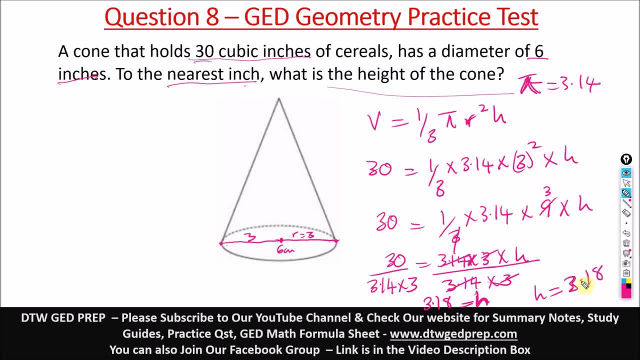 to the nearest inch. so to the nearest inch, you can see here, after the three, after the decimal point, we just have one, all right. one is not up to five, so we can approximate here. so h is just equal to three inches, okay, so this is our answer: three. 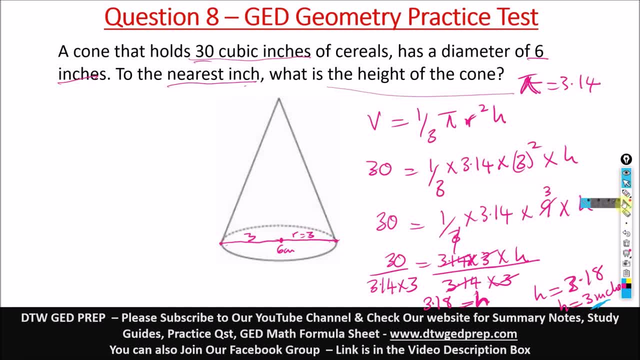 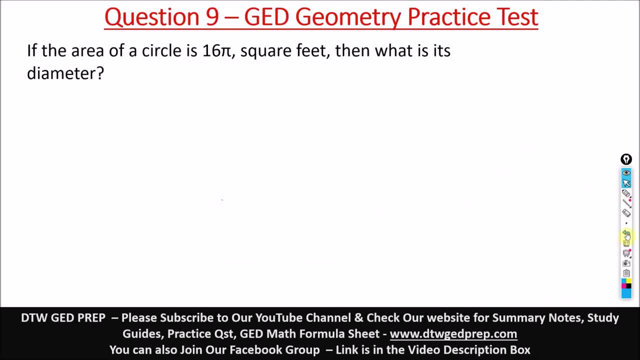 inches. all right, let's go to the next question. so we have question uh, question nine, the ged geometry practice. it says: if the area of a circle area is 16, pi. okay, you can see this now put in pi, all right. so this is not telling us to. this question is not like telling us to. 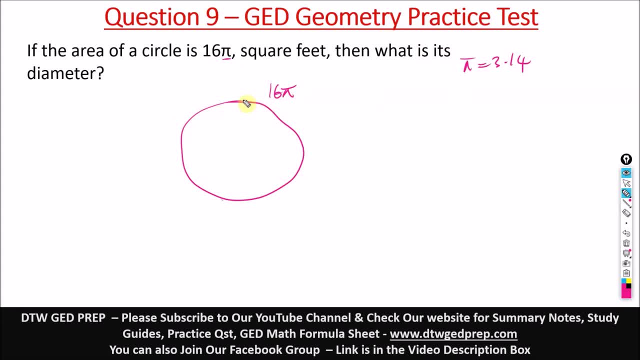 put pi as equal to 3.14. all right, you see what i mean here. if the area of the circle is 16, pi that square feet, then what is each diameter? what's the area of the circle formula? it is: a is equal to pi r square. so the question is asking for its diameter or the area. is this by r square. so we 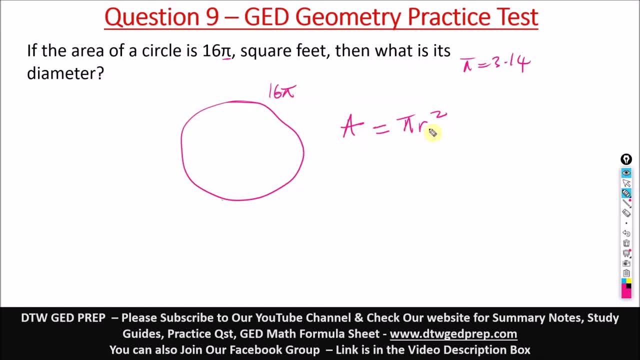 have to look for the radius first. with the value of the radius we can now get the diameter. all right for this. we can look for the radius by the radius. okay, if the area of the edge of the circle is 16, we would get 16 pi bonus. all right. so that's the standard of standard model. so you can see. 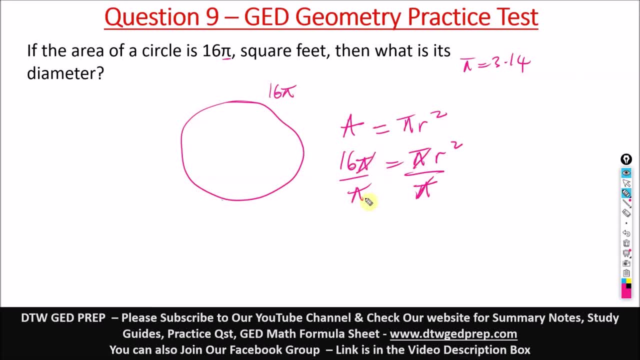 here that we are angering the overall equation. we wanted to calculate the Texas alignment, our frontier area, here. check this right now. all right, we look for the r square here and we align 2 sides with it. make sure you look at this, to make sure. torichスixel and about in two almost equal the area equal to pi, which is 16 pi. 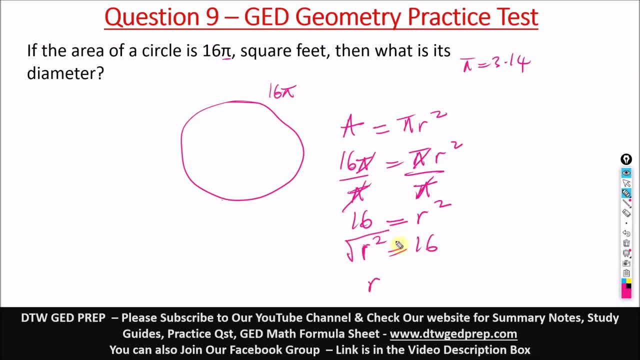 go for spar then so we can easily to mark r square standalone. to get just r, we do what we square root both sides. so when we square root 16 we get 4. all right, so our radius is 4. it doesn't stop there. it says what is its diameter. okay, don't. 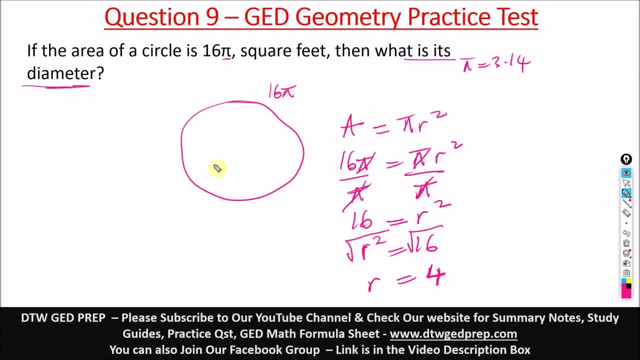 just stop there and just pick the option 4, what is its diameter? so the diameter will be 2 times what d is. 2 times r, okay, 2 times radius, that will be 2 times 4, and which is what 8. so the diameter is. 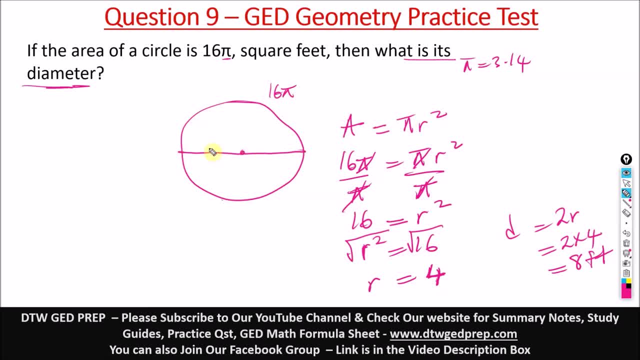 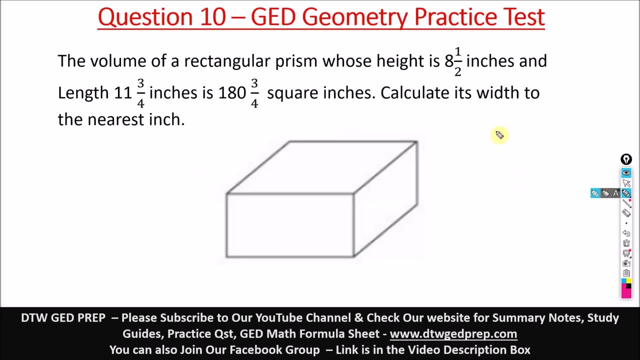 8 feet. that will be the diameter of this circle: 8 feet. all right, so this is our answer. okay, now to the final question here. all right, of our question 10 of the GED geometry practice. it says here: yeah, we have a lot of fractions. it says here: the volume of a rectangular prism. 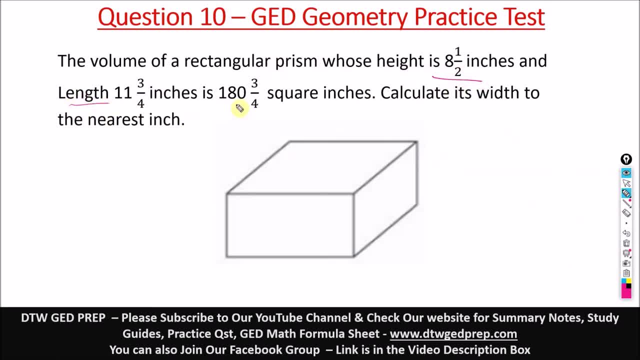 whose height is this and length is this? is this calculated? is width to the nearest inch. now, what is the formula for finding the volume of a prism, rectangular prism? it is v equal to l times what width times your height. okay, so we know our v as this. let us just, you know, put our three over four, as you know points, so this would be 80.75. 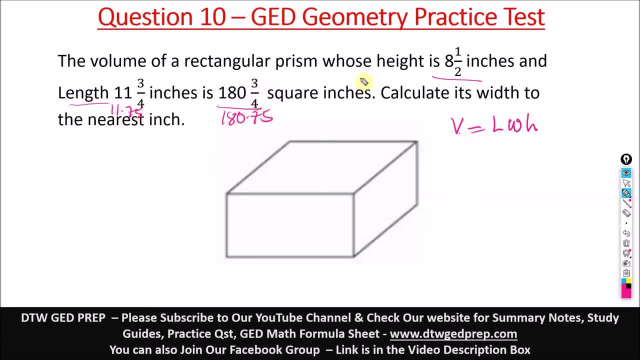 this is 11.75 and our half here is 8.50. okay, so our v volume is 180.75, equal to, are we given our length? yes, our length is, uh, 11.75. we're told to find our width, so the width is the unknown, so leave. 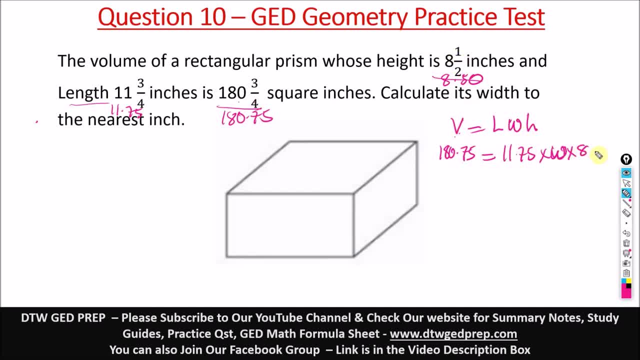 it as w our h is what 8.5 you 0. so from here to get our width standard to make it stand alone, what we'll do is we divide both sides by this: 11.75 times 8.50 times 8.50. so this would cancel out, this would cancel out what left here, with just w when you 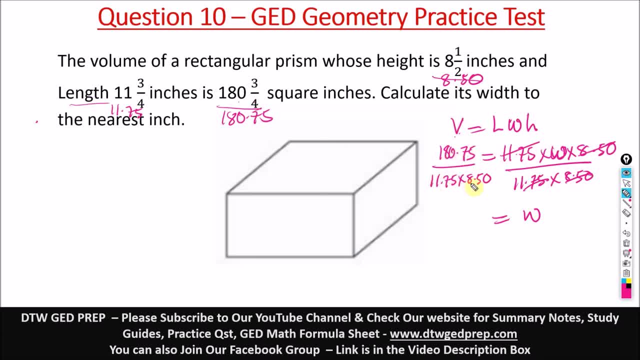 punch in your calculator one, eight. this divided by this times, uh, and this. okay, it would give us what 1.809. so w our, which is what 1.809 inches? okay, but here it says to the nearest, what inch? so to the nearest inch we can approximate this, since immediately after 1 we have a number that 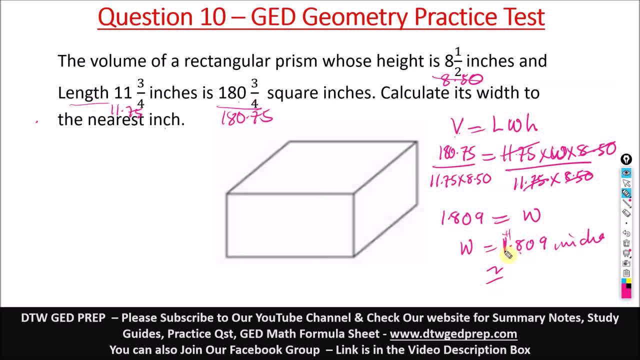 is greater than 5, so we can approximate and add a 1 here. so 1 plus 1 is 2, so our final answer is 2 inches to the nearest inch. okay, so two inches. so thank you for staying tuned to the end of these. 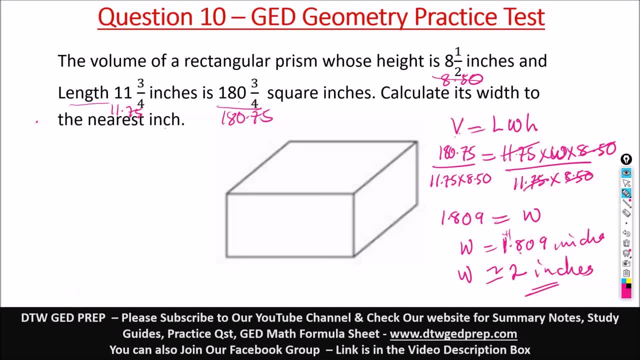 10 questions focusing on the ged um geometry. okay, so i know that as you watch this video to the end, any geometry questions. you know i've done a video on how to find the perimeter and area of irregular shapes and figures. okay, i will leave. all the videos are individual geometry crash course. 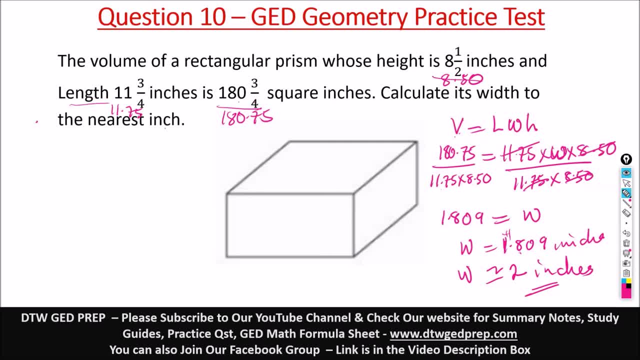 the playlist and also you can get those videos. on my course and after the course there are several practice questions you know you can use to. you know practice and practice and practice. it's needed to pass your ged maths okay. so thank you for staying to the end of this video. finally, don't